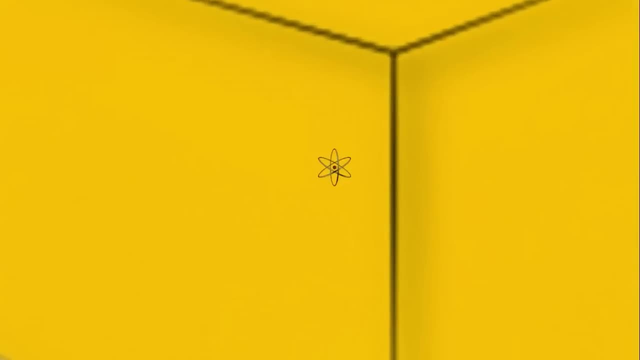 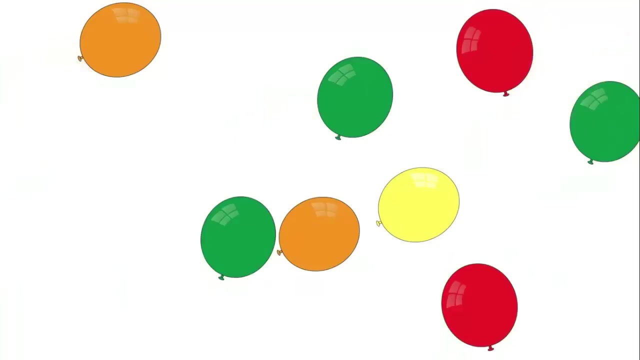 – an individual gold atom. Think of the block of gold as a room of balloons. If you half the number of balloons in the room, half it again and again and keep doing this till you eventually end up with just one balloon and then you cut the last balloon, does it still function as a balloon? No, The same. 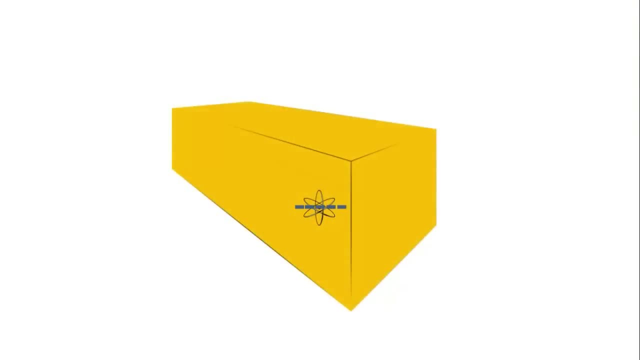 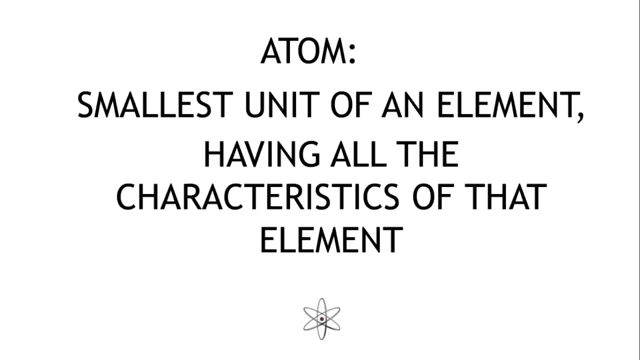 can be said about atoms. If I were to half the last atom of gold, it would no longer be gold. So an atom is the smallest unit of an element having all the characteristics of that element. 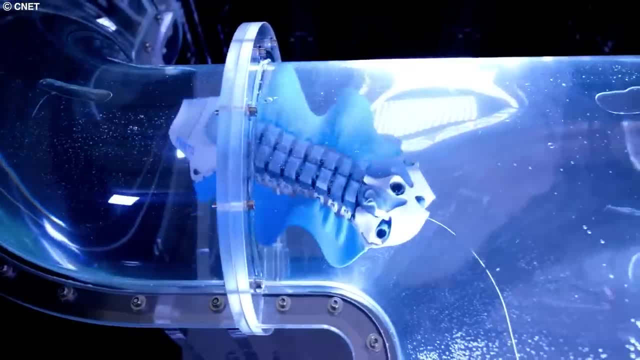 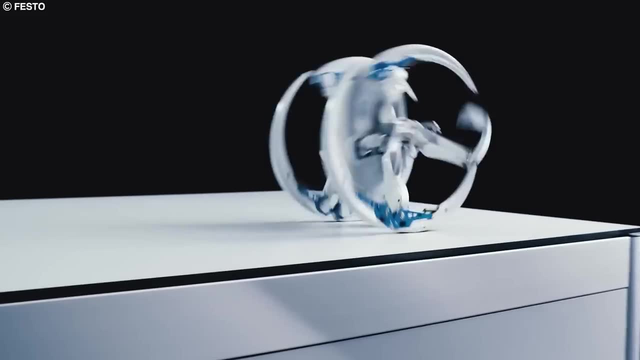 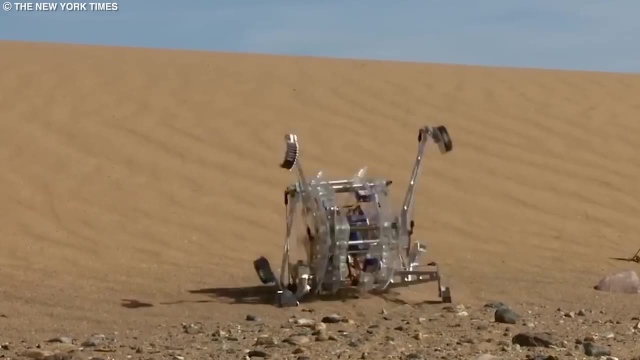 This bionic wheelbot is not only able to exhibit unique movements, it's likewise able to adapt perfectly to just about any environment and traverse even the toughest of terrains. But it's this robotic spy crab that's fast revolutionizing how we study animal behaviors. 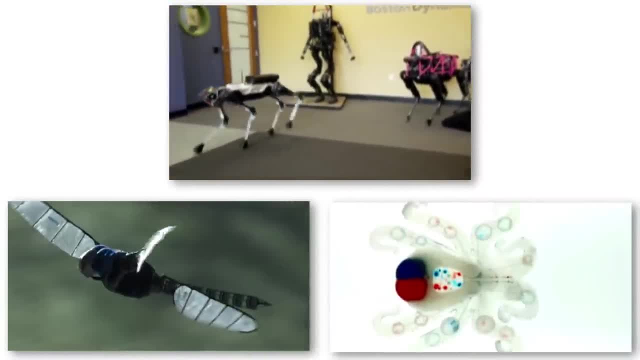 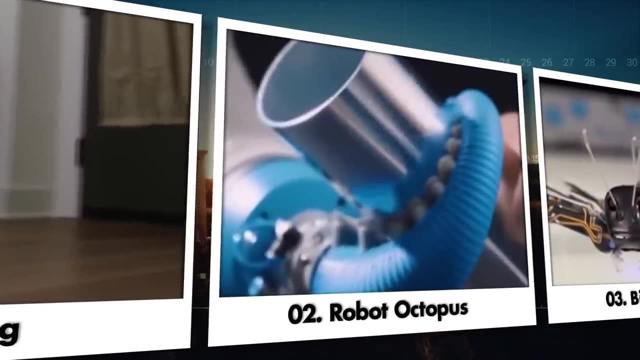 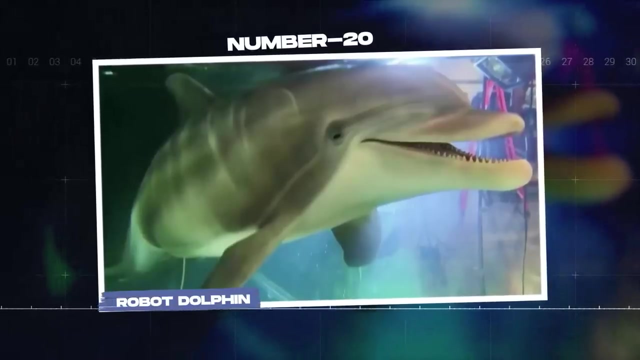 as well as taking our understanding of these crustaceans to unprecedented levels. In this video, we've detailed 20 amazing robot animals that will absolutely blow your mind: 20. Robot Dolphin. Now just imagine walking into SeaWorld and being greeted by not only live animals. 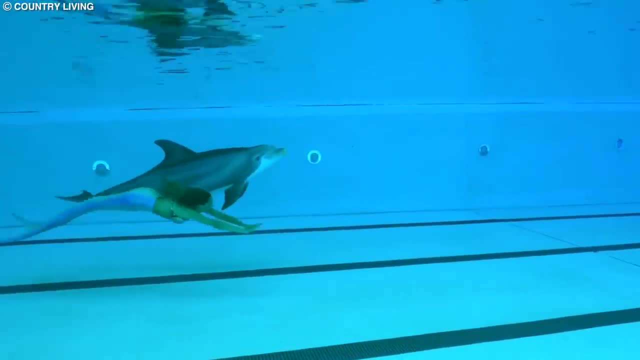 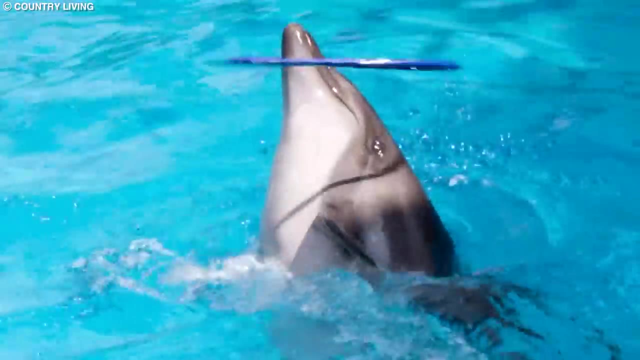 but by a pod of incredibly realistic robotic dolphins, jumping and flipping through the air just like their real counterparts. And while this may seem like a futuristic fantasy, the truth is that it could soon become a reality, thanks to the incredible works of EDGE Innovations. 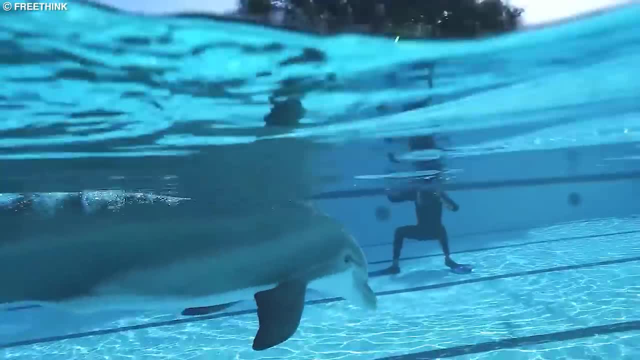 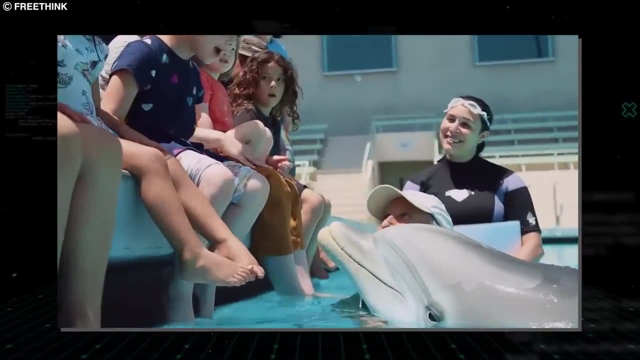 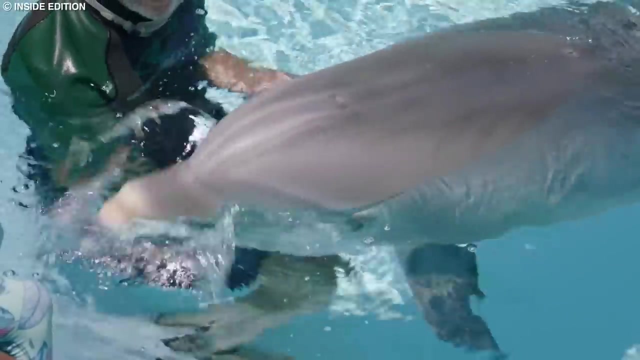 These robots are not only a substitute for their live counterparts. they're also a technological marvel and are already revolutionizing the way we think about live animal shows and marine conservation. Using their advanced AI sensors and programming, they are able to learn and adapt to their environment, interact with humans.